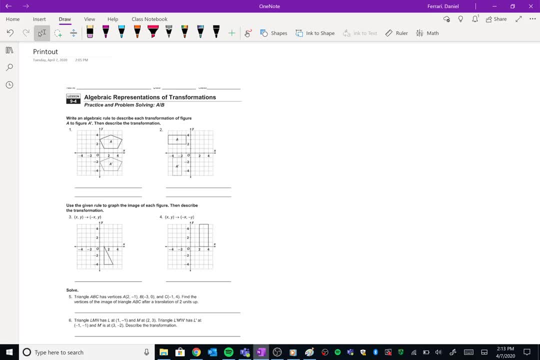 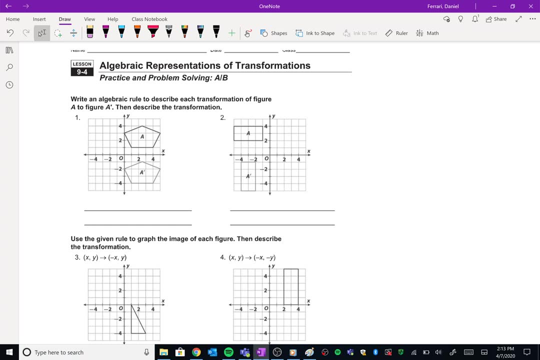 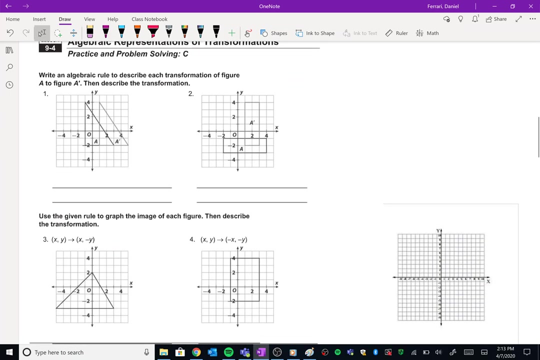 All right, let's go ahead and take a look at 9-4.. So this one is one of the ones out of the textbook pages. So I am going to actually do practice and problem solving C. So if you see, AB, practice and problem solving C is the hardest of the pages. So I'm going to do that one totally. I'm going to do the entire thing And then we'll talk about some of the other pages. But I think by doing this it's going to demonstrate basically most of the pages. 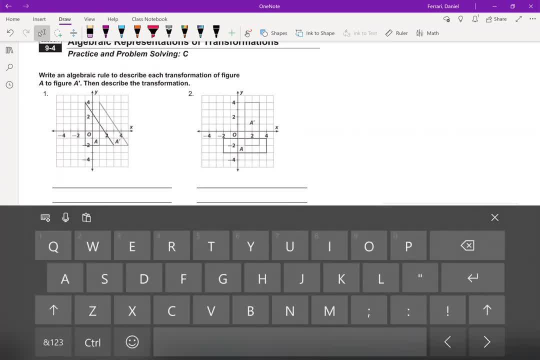 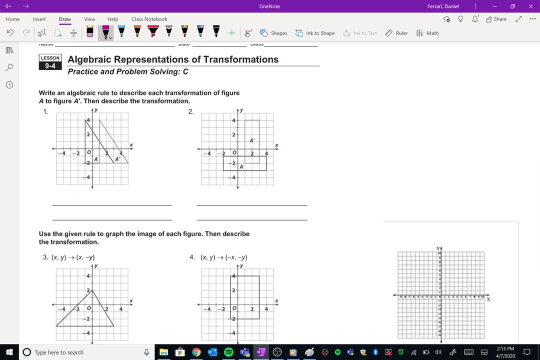 Most of what we're going to need, what you guys are going to need, to be able to do these problems. Okay. so algebraic representations of transformations, practice and problem solving. C. So we're going to be writing an algebraic rule to describe each transformation of figure A to figure A, prime, Okay, and then we're going to describe the transformation. So we got our first triangle, which is A, which is this red triangle right here, Okay, and then, after it gets moved, it turns into: 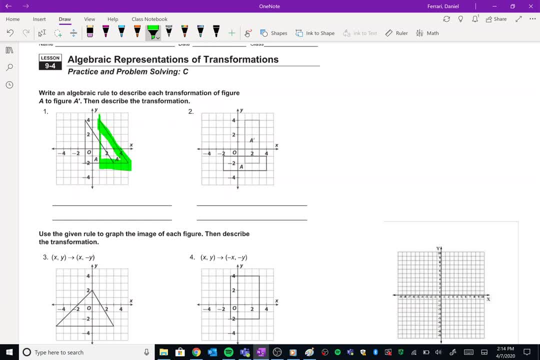 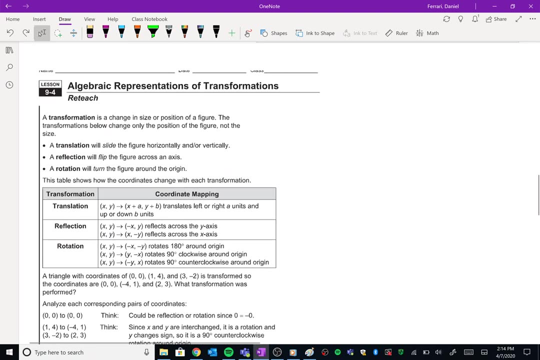 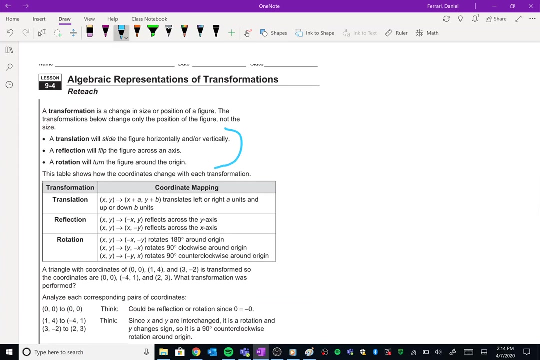 A prime, this green triangle right here. Okay, so essentially, what's happening is, in these problems, you're going to want to identify what type of transformation you're doing, And so remember- and I'm going to switch to the reteach page for just a second, just as a demonstration- Okay, remember that there are basically three types of transformation you're going to look at. Okay, you've got a translation where you're sliding the shape. You've got a reflection where you're flipping the shape. 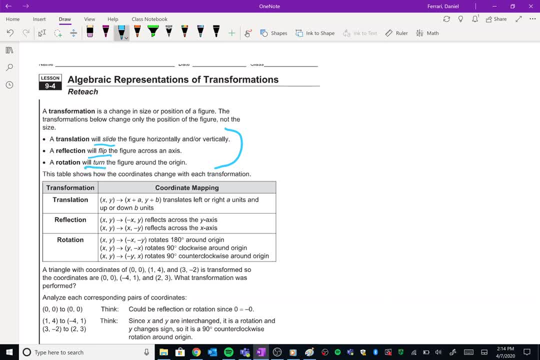 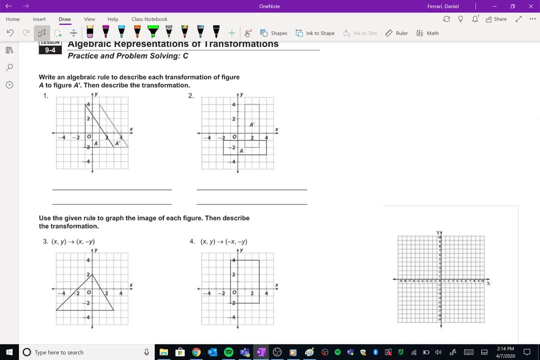 And, finally, a rotation where you are turning or spinning the shape. Okay, so when I go back and look at my problem here, this one doesn't really look like a flip, doesn't really look like a turn right, It's just kind of A is just moving over and becoming A prime. A is just moving over and becoming A prime. You can kind of see exactly what it's doing, Okay. so the trick is, though, is that it wants us to 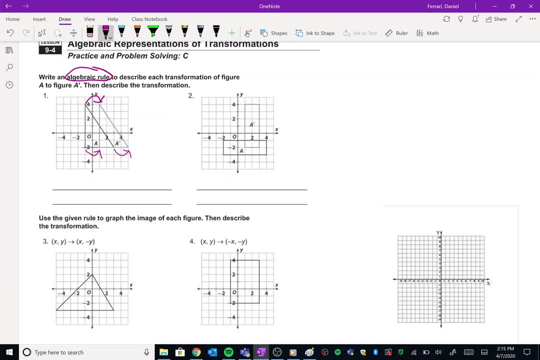 give this as an algebraic rule, So, and it wants to describe it. So I bet you describing it for most of you guys is going to be easier, So I'm actually going to do that part first, Okay, so if we want to just describe the transformation that's taking place from A to A prime, well, that looks pretty simple, right, It looks like it's a translation because it's just a sliding, So we're going to translate two units, right? Okay, as in. 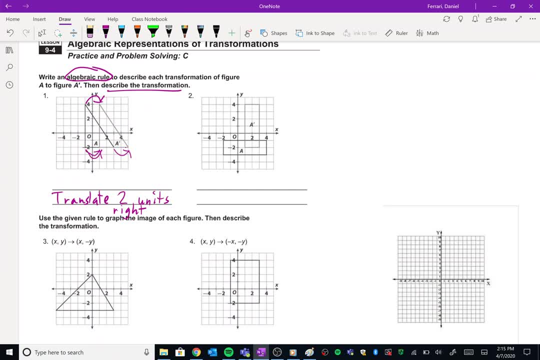 I'm just going to slide it over two units, Okay, All right, let's go ahead and now look at the algebraic rule here. And so the easiest way to do this is to actually look at these points and what changed. So I'm just going to look at these top two points. Okay, so we're going to call this one point A and this one A prime, because that's going to be the. you know, it's the name of the shape, but we could also make it the names of the points. Okay, so for point A, 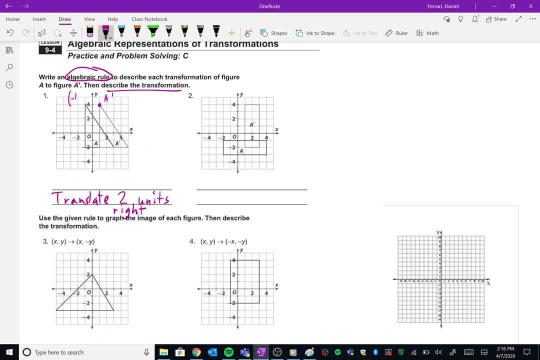 the coordinates of point A are going to be negative, one and four Okay, whereas the coordinates of A prime, on the other hand, are going to be one, four Okay. so you notice, in that the only thing that changed here is my X coordinate, which makes sense, because if you move something to the right, the only thing that's going to change is 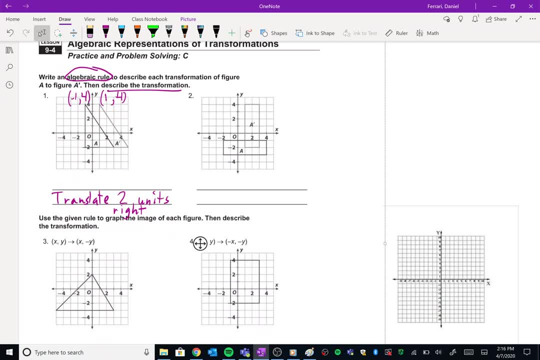 of those points is just the X coordinate, because you're still going to go up four units for the four and the Y coordinate. Okay, so the way we're going to start every algebraic rule is we're going to start it with X comma Y. So it's basically saying, take the first point which is going to be represented by X comma Y, We're going to draw an arrow and then we're going to change these values by something. Okay, so, in this case, what happened to this negative one? Excuse me, What happened to the? 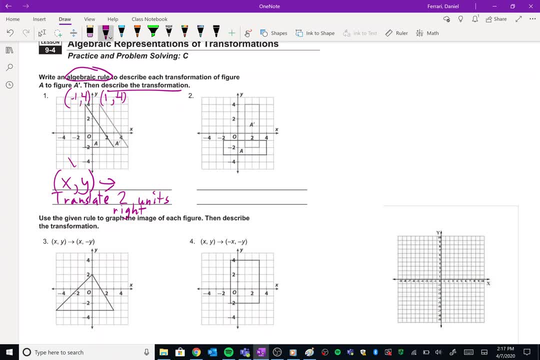 negative one to turn it into a positive one. Well, think about what would you add or what would you do to change negative one into positive one. Well, the easiest way, and what we did in this case, is we added two to the X coordinate and then, for the Y coordinate, Well, we kept the Y the same, So we're just going to write the variable Y, Okay. so essentially what this is saying is: take your X and Y, take the X coordinate and add two to it. 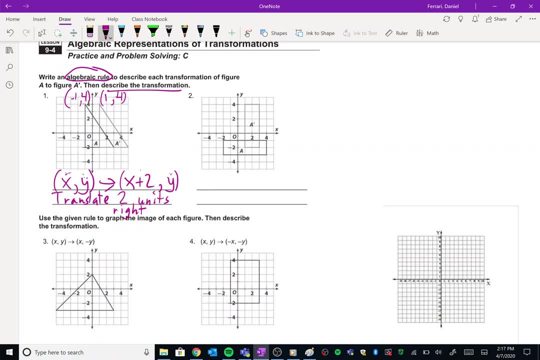 the y coordinate and keep it the same. okay. so, as we go through this, these problems, we're going to be taking something that is in words and we're going to be turning it into something that is algebraic. okay, so let's go ahead and take a look at the next one. okay. so, again, the first thing we 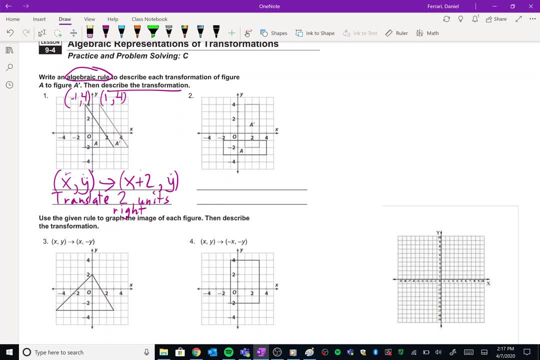 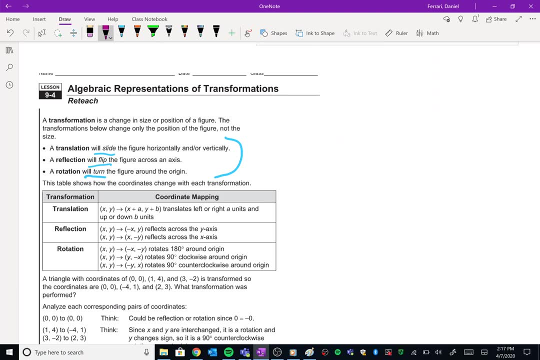 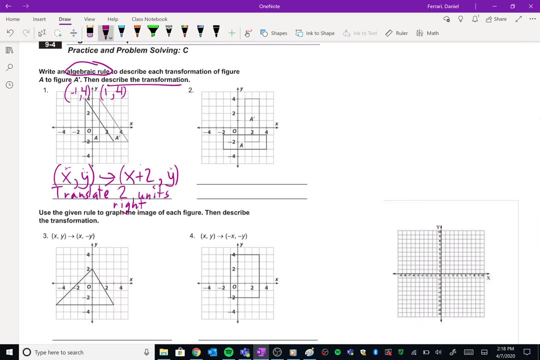 want to identify is: what type of transformation are we looking at? okay, and remember again, our choices are: we can have a translation which is a slide, a reflection, just a flip, or a rotation which is a turn. well, this one's definitely not a translation. okay, it doesn't look like we just 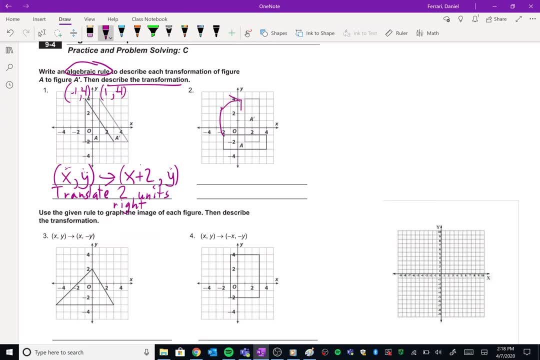 slid a up into a prime. that wouldn't work, because that would be. we would end up with a rectangle that looks like a that's kind of on its side, like that right, and we want a rectangle that's tilted, a rectangle that's up on its side. okay, similarly, reflection probably. 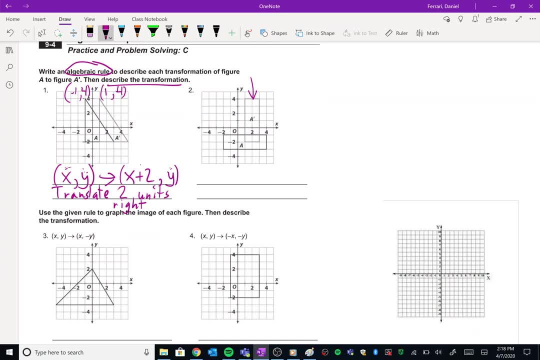 isn't the greatest here either. okay, because it doesn't really look like it's being flipped over any particular line, and it's definitely not being flipped over like the x axis or the y axis, which makes our life a lot easier. if it's a reflection, okay. so instead this one is going to be a rotation. 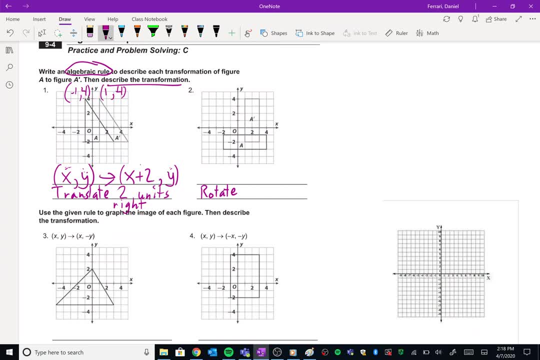 okay, so we're going to rotate this one. now, how do I make a into a prime? well, you know, if you're on paper, this is pretty easy, but you're going to take your shape and you're going to rotate it up to a prime, okay, so sorry if you heard my dog there, someone's at the door, okay. so how much am I? 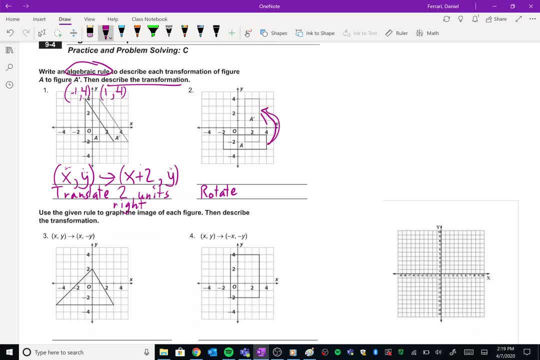 rotating to get from a to a prime. well, this looks to me like a 90 degree turn. okay, it's a. it's moving from the fourth quadrant down here up into the first quadrant, because it's only moving one quadrant over. that's going to be a rotation of ninety. 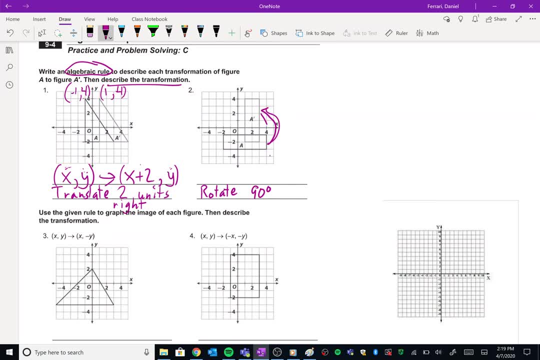 degrees. okay, now that rotation of 90 degrees. remember, because it's 90, we need to give a direction. okay, so my arrows appear to be going counterclockwise, so please make sure if you're going to do any sort of rotation where the direction matters, so, for example, like a 90 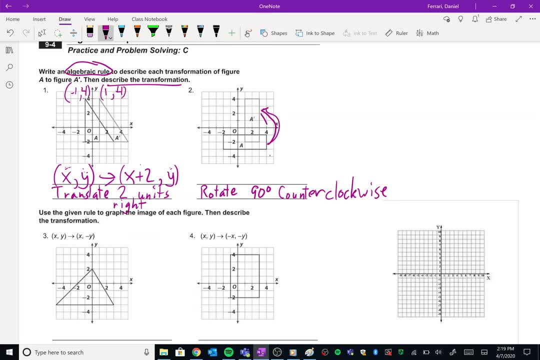 degree rotation or a 270 degree rotation. be sure to tell us which direction you're rotating it, because that's going to matter. right? if you said 90 degrees clockwise, you're going to end up over here, okay, we want to end up counterclockwise, so back that way, okay, all right. so now again, I'm going to pick out two points that 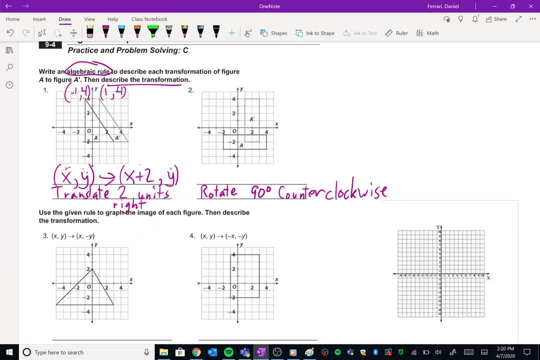 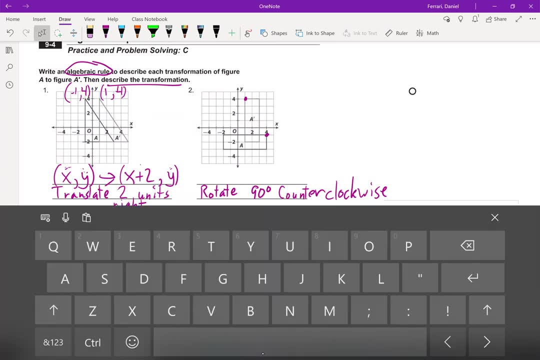 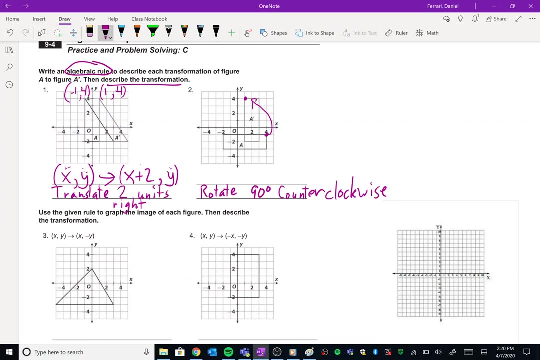 correspond with each other. okay, so my easiest ones look like here: I'm going to use this point and this point. okay, and the reason why I'm picking those two is because that's where that point will end up after I do the rotation. okay, because this one's the top right, and after I rotate it: 90. 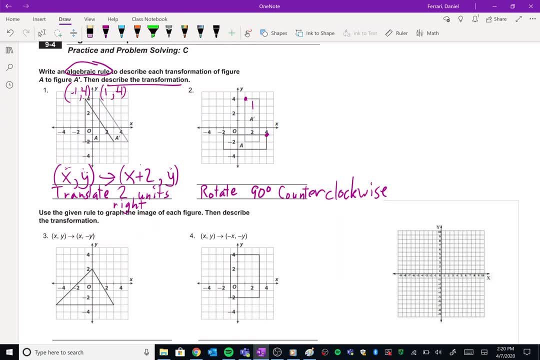 degrees. it's going to end up up here, okay, so, okay. so now let's look at the coordinates of this point. so, for point a, this one is four negative one okay, and this point is one four okay. so this is something you want to be paying attention to notice that these numbers are very 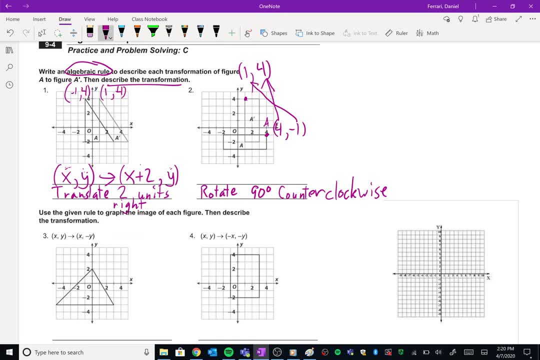 very similar. I still have a 4 and a 1.. Now, granted, the 1 has turned from a negative 1 in point A to a positive 1 in point 1, and we're going to talk about that one in just a second okay. 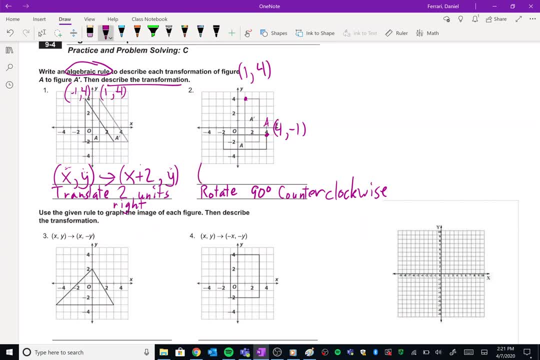 But so let's just track this as we go. So, like I said before, every algebraic representation is going to start the same way, with x, y, because basically that's just saying, take your first point and do something to it. okay. 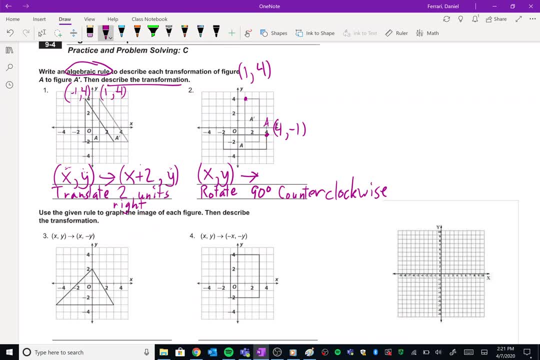 So they're always going to start with x, y, Okay. so now, what did we do with the x-coordinate? So before the x-coordinate was 4, okay. Well, now the x-coordinate is in the y-spot. So that means, in my point, 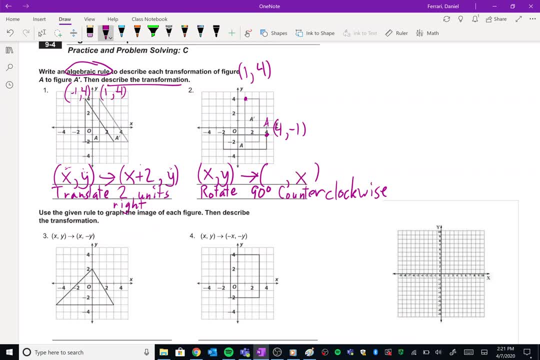 I'm going to end up with x in the y position, So notice how x has now moved to the back part of the point, because it is now representing the y-coordinate for my point, okay. Similarly, the y-coordinate has also switched sides. 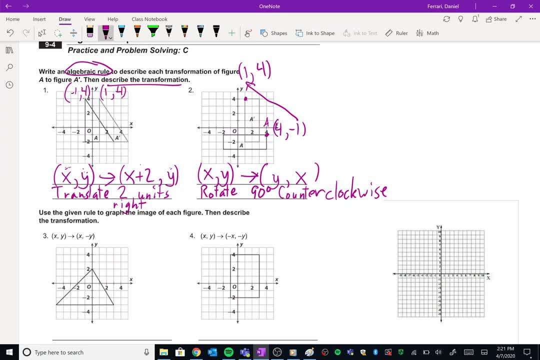 So I know that I'm going to put a y in this first spot, okay, But right now I'm not done because according to this transformation, the point 4, negative 1 would turn into negative 1, comma 4,. 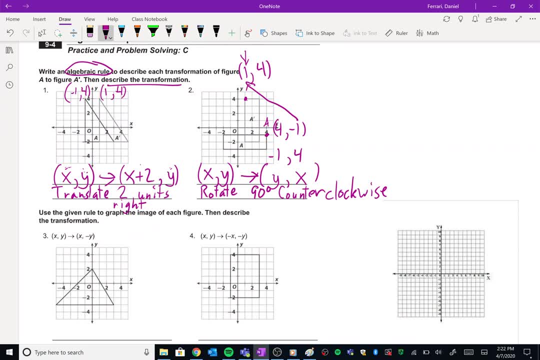 and that's close. but remember, I want this to be a positive 1, okay. So how do I make a negative 1 into a positive 1?? Well, that's pretty easy. All I have to do is make the y-value its opposite: make it negative, okay. 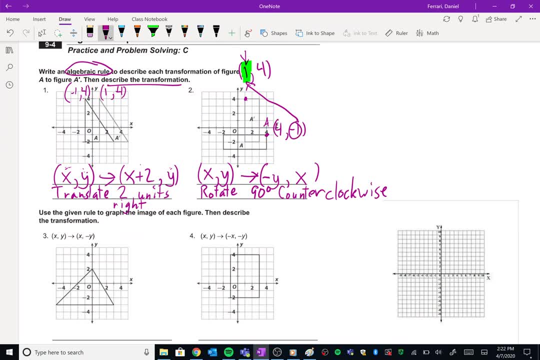 So if I take this negative 1 and I turn it into a positive, now I've got my transformation. So x comma y translates or- sorry, excuse me, rotates into negative y comma x. okay, And you'll notice, because those coordinates switched. 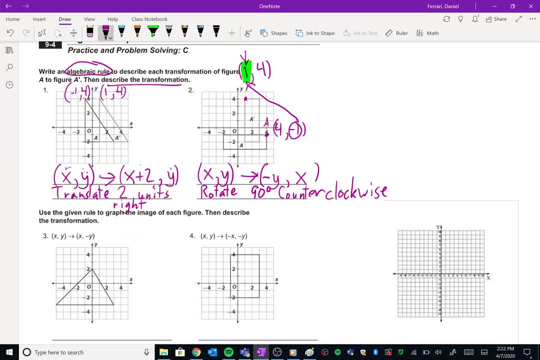 that's what causes the rotation, okay. So really, what we're doing here is we're taking something visual and we're turning it into something that is algebraic. We're turning it into symbols, okay. So every time you do one of these, 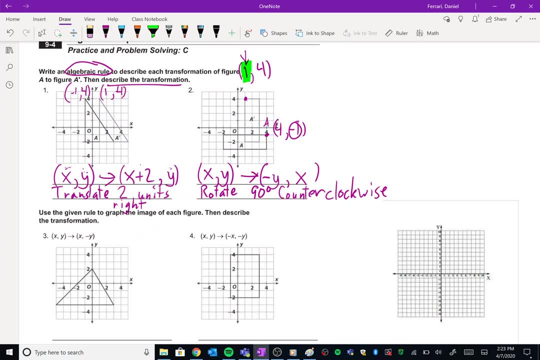 I want you to start with the coordinates and work from there, okay, So when you're trying to come up with the algebraic rules, look at the coordinates and compare them- What changed, What stayed the same- And then set up your rule accordingly. 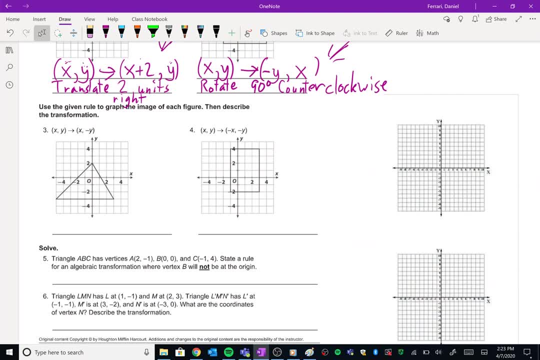 Okay, let's look at number 3 and number 4.. So this one they're giving me the rule. okay, They're saying: start with your point x, y, make x stay the same. So my x coordinate's going to be consistent throughout this. 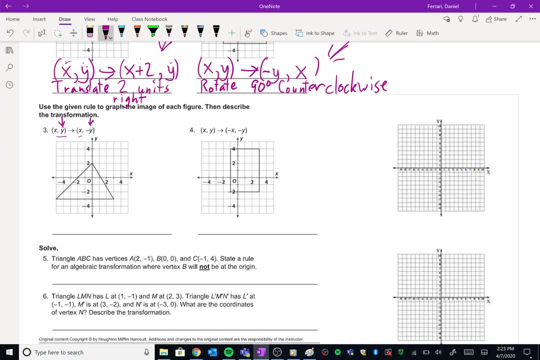 but my y coordinate will switch to its opposite. okay, So let's take a look at one of these coordinates and see what we have. So, for example, this point: okay, So I'm going to label these with letters, real quick. 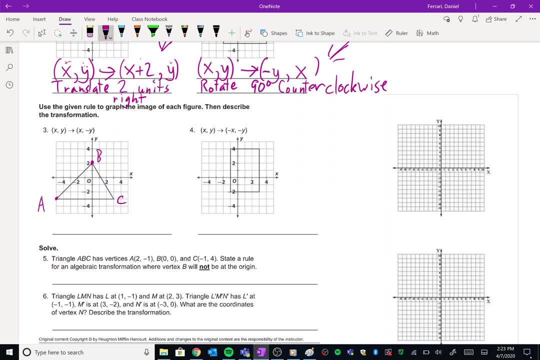 just to make my life a little bit easier. So a, b and c. So let's start with point b, okay, Point b has the coordinates. Okay, so notice how, if we follow this rule, my x coordinate will stay the same. 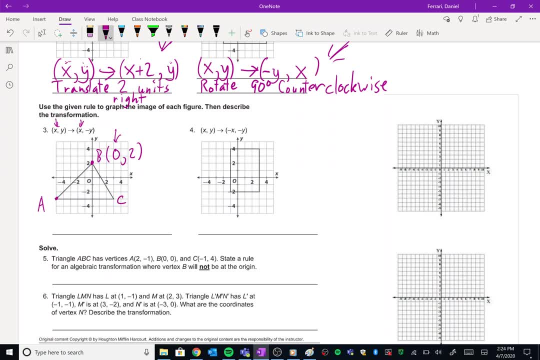 So that means the 0, so when I do b prime its coordinates, the x coordinate will be 0, okay, And the y coordinate, on the other hand, we're going to take the y and we're going to make it its opposite. 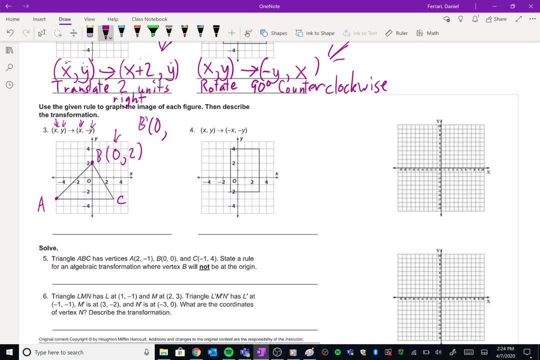 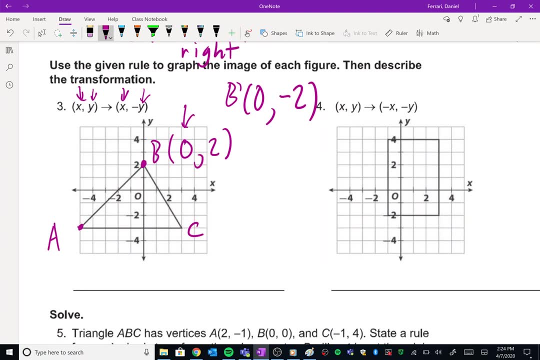 We're going to make it its negative, okay. So the negative of positive 2 is negative. So the y coordinate is going to be negative 2, okay. So now, if I plot that point, I'm going to zoom in just a little bit. 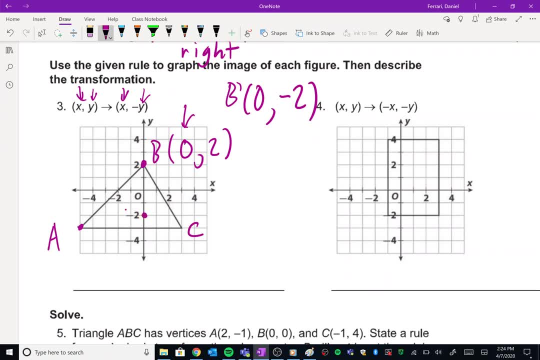 to make this a little bit clearer. okay, I'm going to plot the point in 0, negative 2, and this is going to be point b. okay, B prime, excuse me, Okay, so now we're going to repeat that process for the other points. 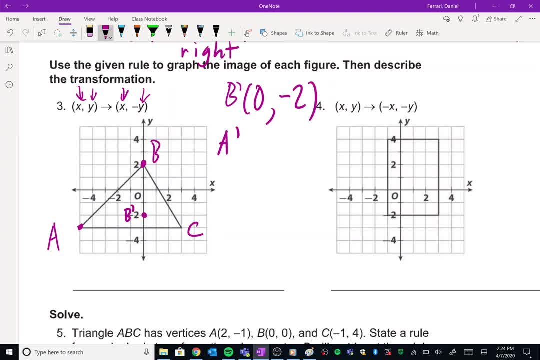 So let's look at a prime. So the first thing we want to do before we can do a prime is we need to get the actual coordinates. So a is going to be negative 5, and I go left to 5, and down 3.. 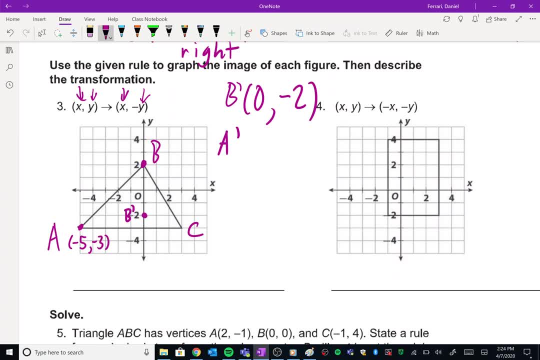 So negative 5, negative 3, okay, Again, follow our rules. The x coordinate stays the same and the y coordinate becomes its opposite. Well, what is the opposite of negative 3?? What's the negative of negative 3?? 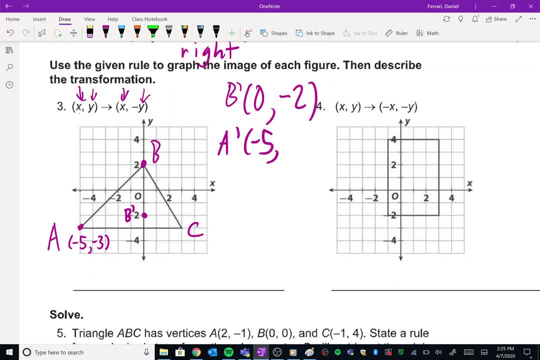 Well, if you remember back to our integer work, a negative times a negative is a positive. okay, So that means it's negative 5,, positive 3.. So now let's plot that point: Negative 5,, left to 5, and then up 1,, 2,, 3.. 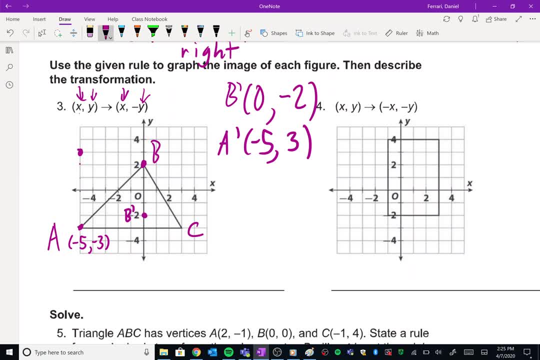 I'm going to plot our point right here, and this one is a prime, okay. So now, if I start to connect- oops, excuse me, my Spotify's coming up- okay, If we start to connect our points, we have one last one to do. 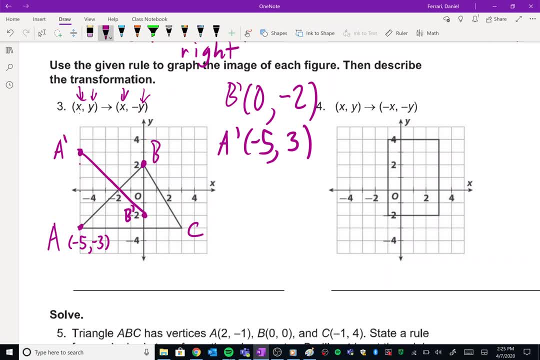 but now you might be able to start seeing the pattern, right. Well, what happened to b and a? Well, it looks like they flipped. It looks like they flipped over this middle line, which is the x axis. okay, So if we look at this now, if I wanted to, 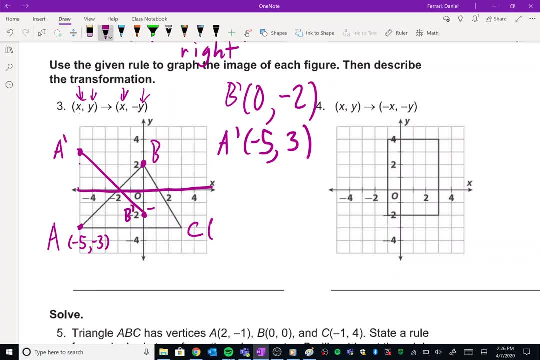 I could just do it the old-fashioned way. I could say that point c is the point 3, negative 3, and then go through and actually figure out what c prime is. Remember the x would stay the same and the y would be the opposite. 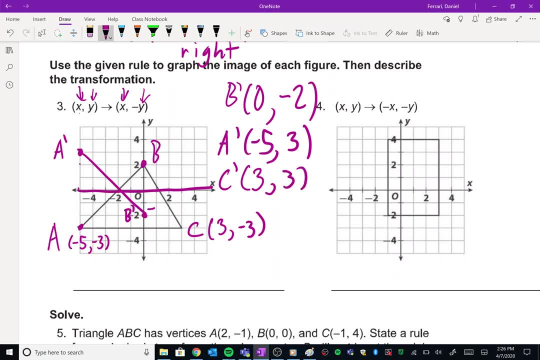 So negative 3 would turn into positive 3.. Go to plot my point and I end up 1,, 2,, 3, somewhere up here. okay, And now. if you didn't see it before, you will definitely see it now. 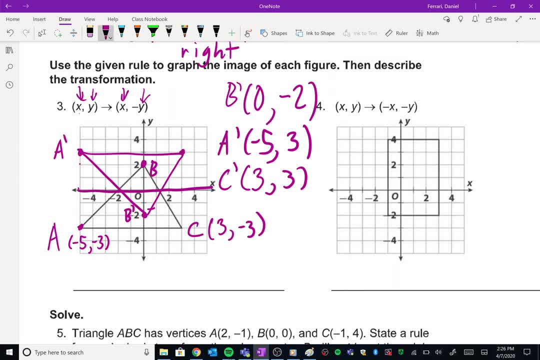 I'm going to move this out of the way. okay, My triangle has now flipped over the x axis. okay, And if you remember, what do we call a flip over the x axis? That is a reflection. okay, And remember when you say reflection. 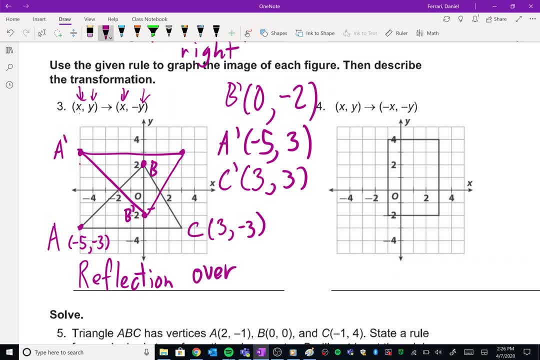 you need to say over what line you're rotating. you're flipping it over, excuse me. So this is going to be reflection over the x axis. okay, We've got one more to do here on this section, So this one again is going to be very similar. 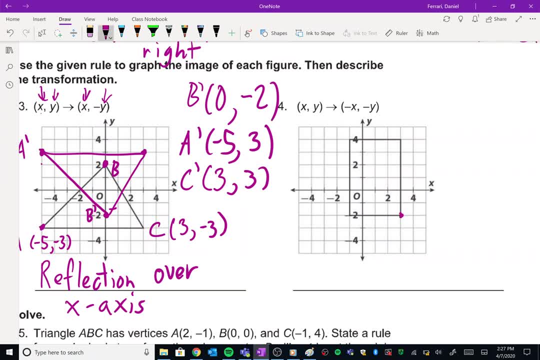 So the first thing I'm going to do is we're just going to plot the. you can just figure out what these points are. So this is 3, negative 2.. And this is negative 1, negative 2.. And this is negative 1, 4.. 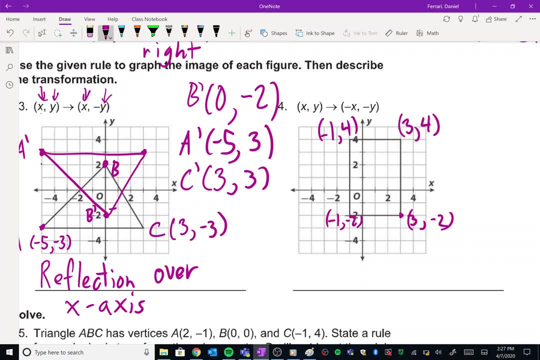 And finally 3, 4.. Okay, so this one has us taking the points and just making them the opposite on both. okay, So both the x coordinate and the y coordinate will turn into their opposites. okay, So I'm going to do these one at a time, okay. 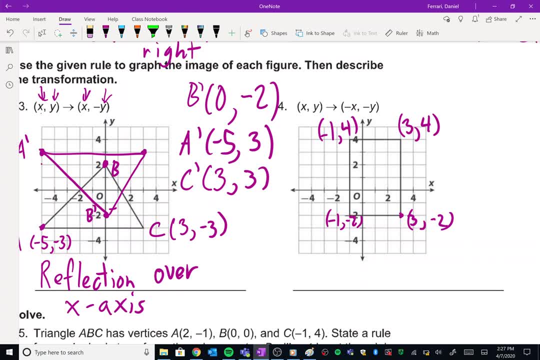 Let's just take the first one. We're going to do 3, 4,, okay, So 3, 4,. when I turn them into its opposites, it's going to be negative 3,, negative 4,, okay. 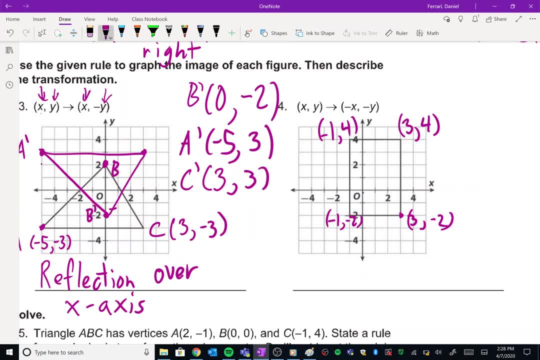 And if I plot that point, negative 3,, negative 4, that's going to put me somewhere down here. okay, As I do these, I'm going to remove the work or remove the previous point, just so I can kind of keep track of which ones I've already done. okay. 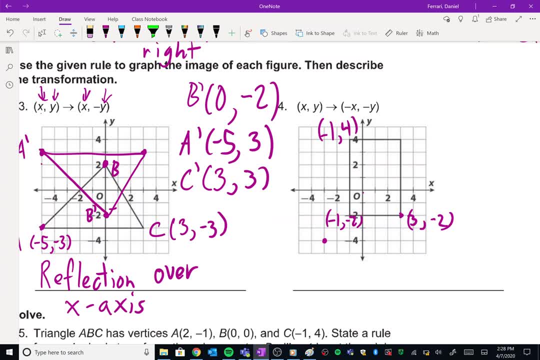 Because one thing that can be a little bit tricky here is: there's lots to do in these problems. It's not particularly difficult, but you want to make sure you're keeping track of everything you're covering. If you wanted to label your points, you could do that as well. 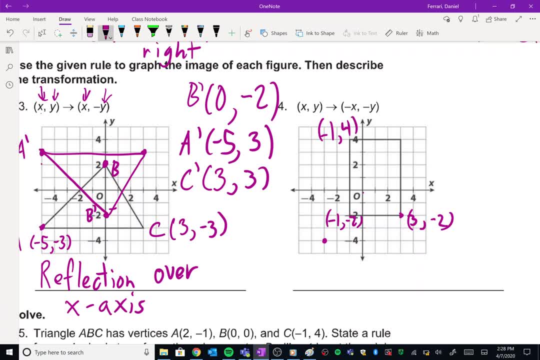 This one's going to be a little too cluttered if I do that, but you can feel free to do that on your paper, okay. So for the next one: 3, negative 2.. Well, the opposite of 3 is negative 3,. 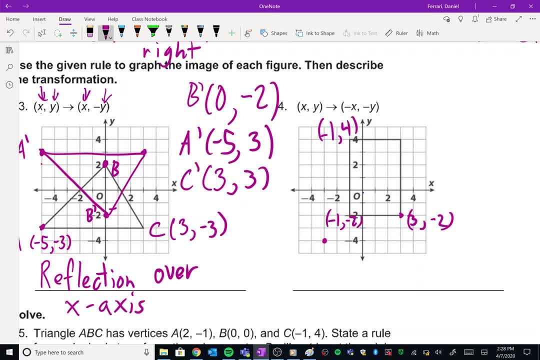 and the opposite of negative 2 is positive 2.. So negative 3, positive 2, is going to put me somewhere about right here. Okay, Our next point: negative 1, negative 2,. well, when both those negatives become their opposites, 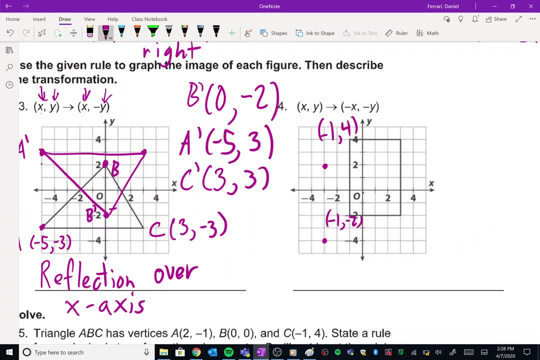 they're going to turn positive, So that's going to be positive 1, positive 2.. I'm going to plot that point up here, okay. And finally, positive 1, negative 4, it's going to put me somewhere down here, okay. 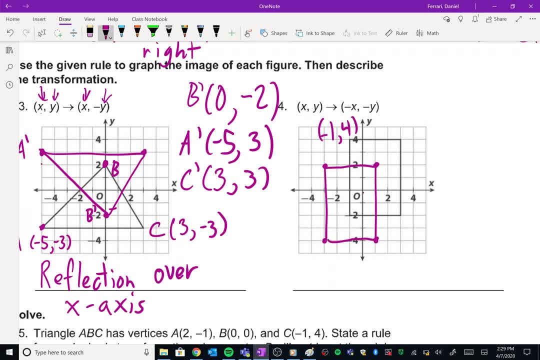 So this problem now what transformation we're doing here- we could actually probably answer this one in a few different ways. okay, And you might be wanting to say this looks like a translation, Mr Ferrari, because it looks like we're just sliding it. 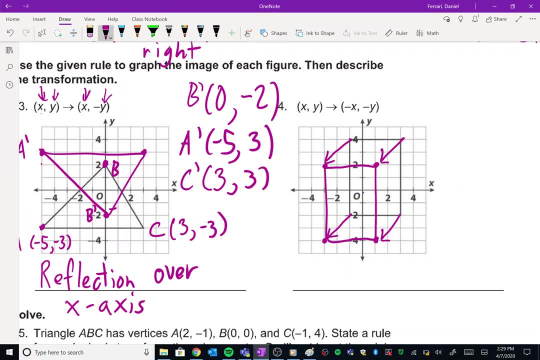 two units down and two units left, And that is true. You could describe this transformation as a translation, as a slide, okay, But it turns out that actually, what we've just done, okay, this thing that we've just done here, is actually the transformation. 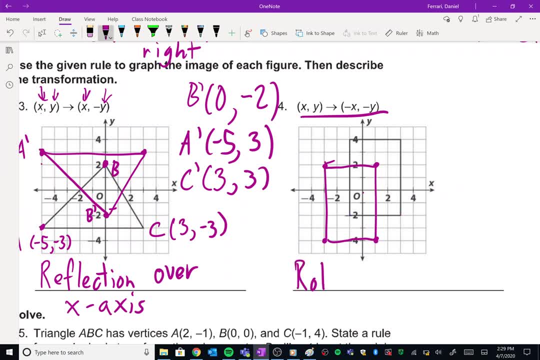 for a rotation. okay, This is a rotation of 180 degrees, And if you notice, that's going to end up in the exact same spot, right, If you take that original printed rectangle and you turn your paper upside down, you will end up with the rectangle that I just graphed. 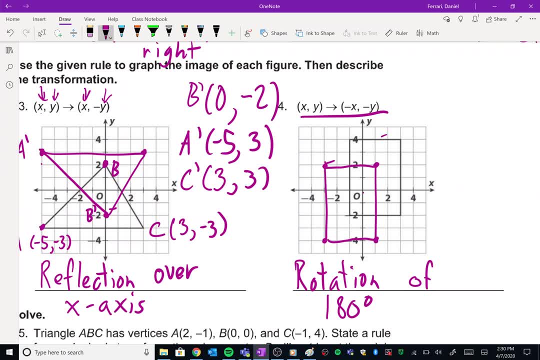 the purple rectangle. okay, So that is going to be a rotation of 180 degrees? okay, If this one had been a translation, instead I would have seen x, y, and then it was left 2 and down 2.. 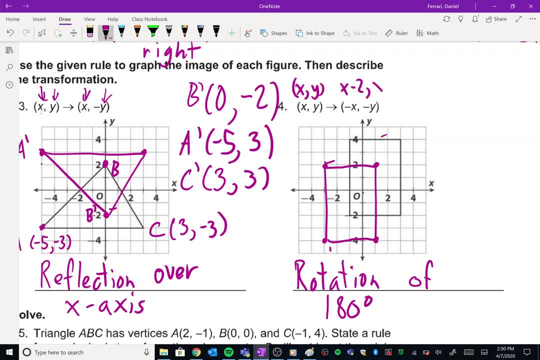 So it would have been x minus 2 and y minus 2, okay, But that's not what we saw, And so in this case, because of that, it would be equivalent, but it would not be the exact answer we're looking for on this problem, okay. 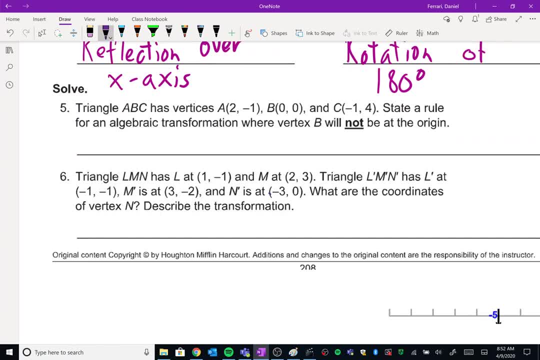 Because this one should be a rotation. Okay, so we've got two left to do. These are number 5 and number 6,. okay, And then these ones. these ones are a little more, or at least for number 5,. 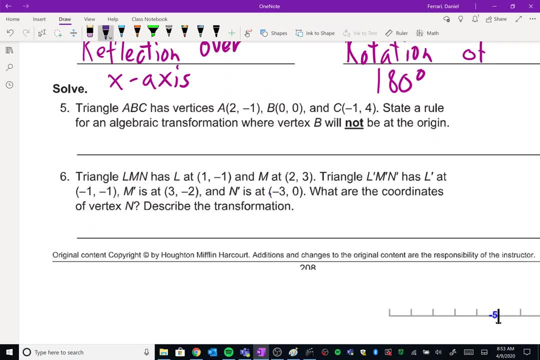 is a little more kind of open to us, okay. So it says we have triangle ABC that has vertices at 2, negative 1,, b at 0, 0, and c at negative 1, 4.. And we want to state a rule for an algebraic transformation. 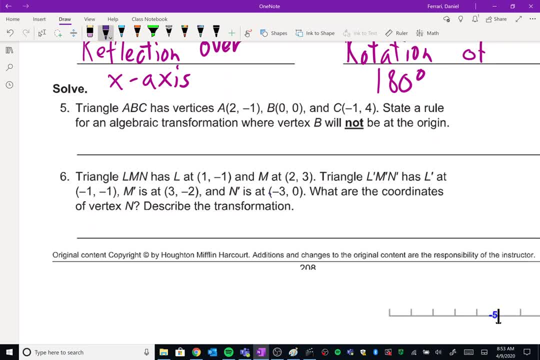 where vertex b will not be at the origin. okay. So the best advice I can give you on a problem like this: if you ever see a problem that doesn't already have a graph, give it a graph. okay, Because it's going to be pretty hard for most people. 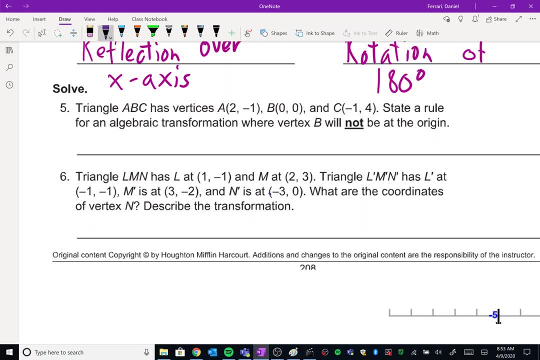 I don't want to say everybody, but for most people to be able to visualize this without actually graphing it, okay. So if you don't have graph paper, that's okay. Just feel free to you know if you sketch it. 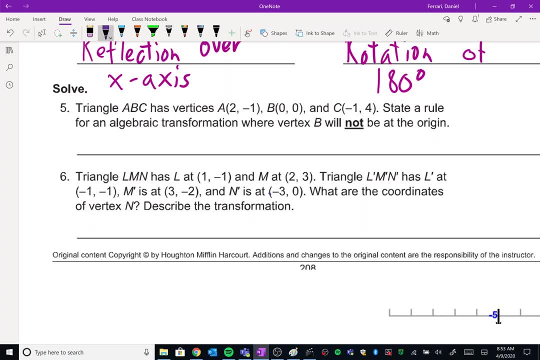 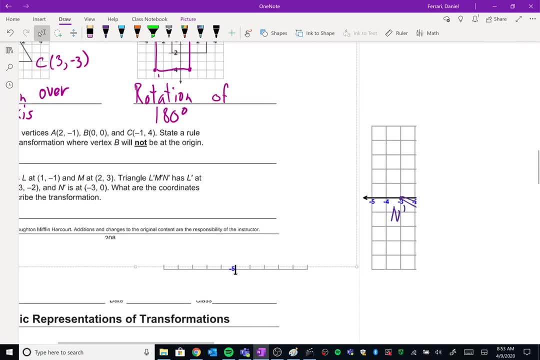 these numbers are pretty small. Just, you know, keep your lines as straight as you can, and you probably can do it even if you don't have graph paper. okay, But I went through just for the sake of being able to describe this problem. 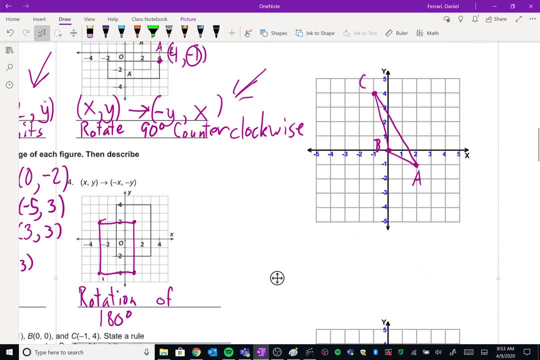 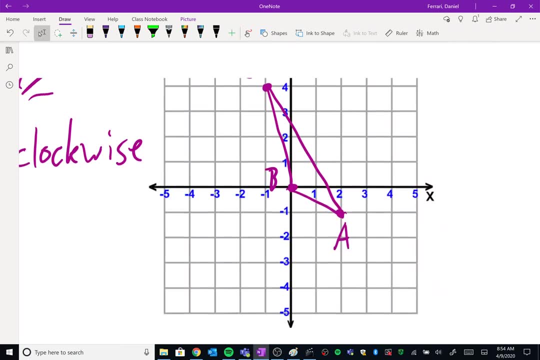 I went through and I actually graphed this guy up here. okay, So we are looking for a transformation that will make it so that this point- ooh, my computer is struggling a little bit this morning- that this point b doesn't. 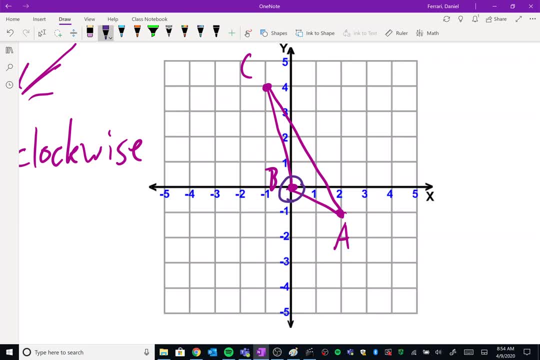 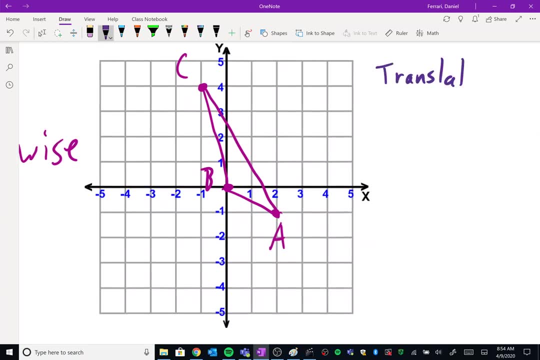 sorry, is no longer at the origin. okay, So, and if you remember back, we have three types of transformations for this section anyway: We have translations, we have rotations and we have reflections. okay, Now, if you remember. 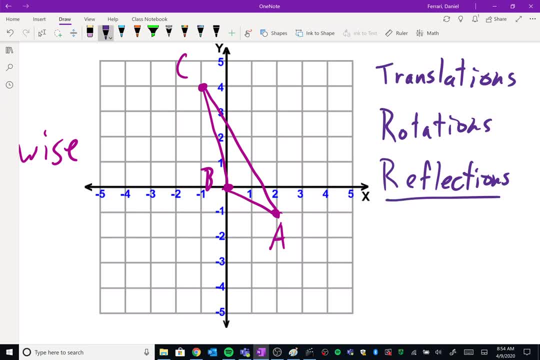 I'm gonna do these kind of in reverse order, okay. So reflections, those are a flip and traditionally they are a flip over a line. okay, And most of the time when we do reflections we do them either over the y-axis. 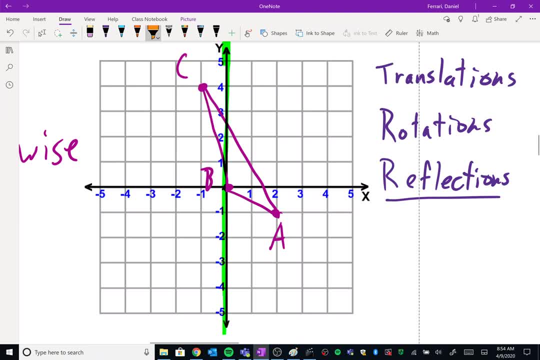 or we do them over the x-axis, okay. Now take a look at point b, though. if you were gonna reflect over either the x-axis or the y-axis, Well, remember that it's sitting right on both. It is on the x-axis and on the y-axis, okay. 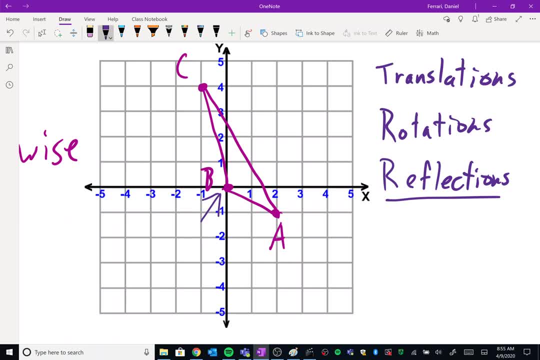 And that means that if I were to do a reflection over that line, that point b wouldn't move. Point b would stay exactly where it is at the origin. okay, And that is not what we want. So there are some reflections that exist. 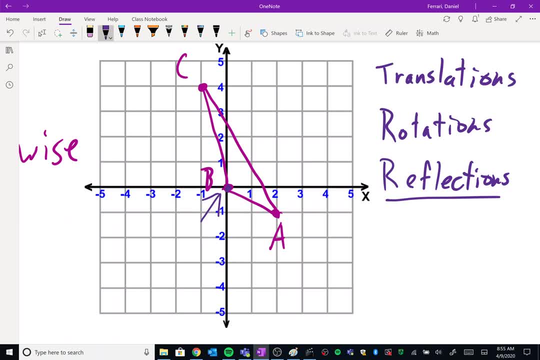 that would make this one not be on the origin anymore. okay, But for our purposes, a y-axis reflection or an x-axis reflection would not work for us, okay, So I'm gonna eliminate that one. okay, Now for rotations. similarly. 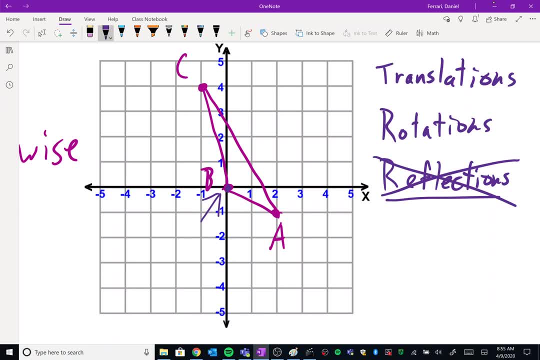 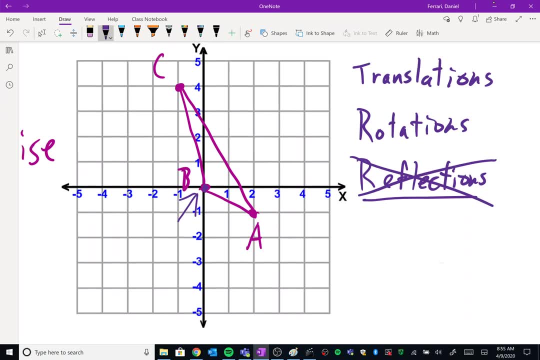 now we have lots of different kinds of rotations. We had 90 degree, we had 180, we had 270.. We could go clockwise, counterclockwise, right, With all of those, okay, But we always did our rotations around the origin, okay. 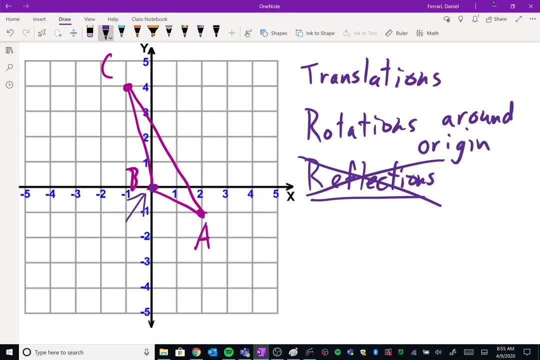 Or in other words around exactly where point b is okay. So if the points are spinning around the origin- well, kind of similar to the reflection one- What's gonna happen to point b if I rotate around the origin? Well, the short answer is it's not gonna move as well, right? 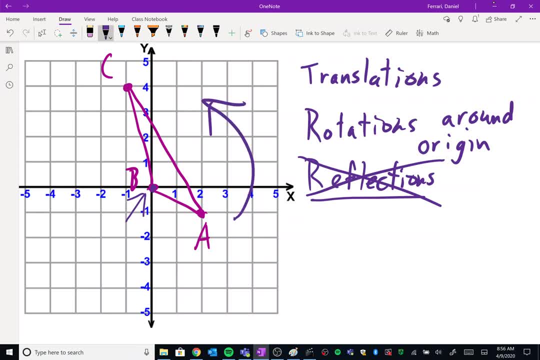 Because it's the point that everything else rotates around, So it stays in place, okay. So that means that, unless we were gonna rotate around a different point which is harder for us to do, okay, it's not normally something we deal with, okay. 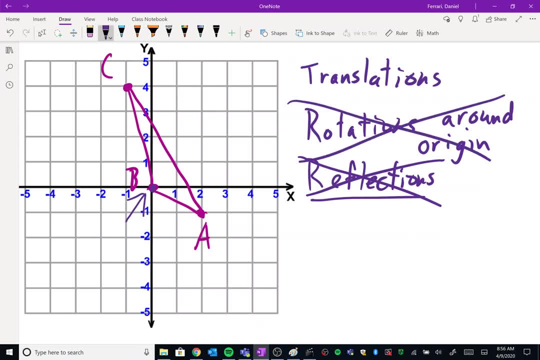 A rotation, in this case at least one around the origin, will not work in this case. okay, So that leaves us with our last one. So obviously our answer has to be a translation And, honestly, translation kind of makes the most sense anyway, right? 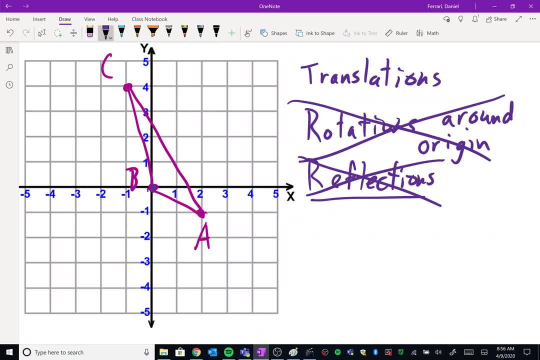 If my only goal is to move b somewhere else. well, what if I just translated it down, let's say, two units, okay? Well, if I slid b down two units and made this b prime? well, now that would be. 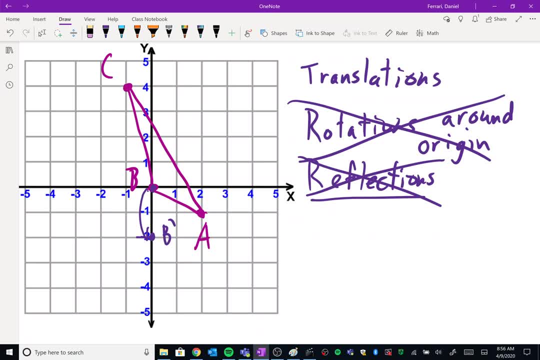 b is no longer at the origin, okay, So any sort of translation will work for this one, So you could feel free to use mine. a translation of down two, You could go down three and right four, You could go up ten. 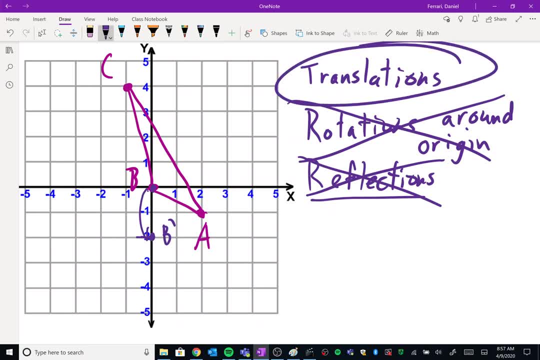 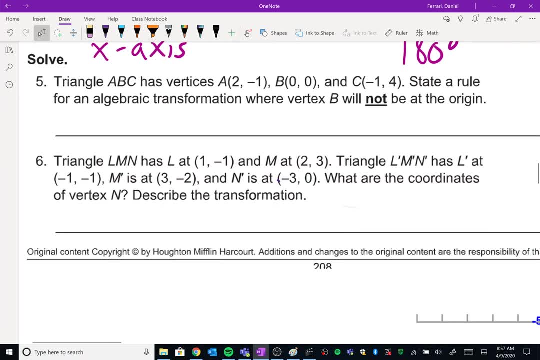 You could do whatever you wanted, as long as you do some sort of translation on this one, okay. So I'm just gonna put that in here, Because it does want it, though as an algebraic transformation, okay. So think back to what we talked about before. 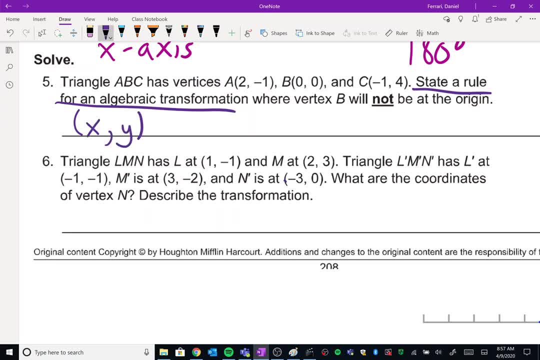 We always, when we do an algebraic transformation, start with x comma y, because, remember, that's the point we're starting with. okay, And then I said for mine that I wanted to move it down two. okay, So, if you remember, if I'm going down, 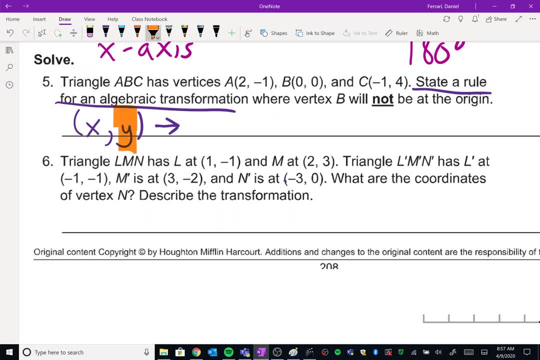 the only coordinate that's gonna change is my y coordinate. okay, So I'm gonna write in my x coordinate just as it is, and then I'm gonna put y minus two, okay, And again all that means that minus two at the end. 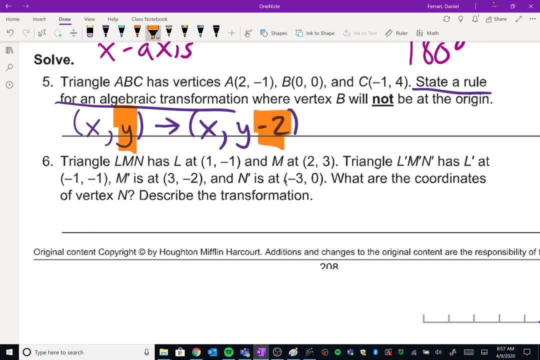 just says: take my y coordinate and bring me down two units, okay, So let's go ahead and take a look at our last problem, which is number six. okay, And again, just like before, I did graph this one, and I would recommend you guys do this as well. 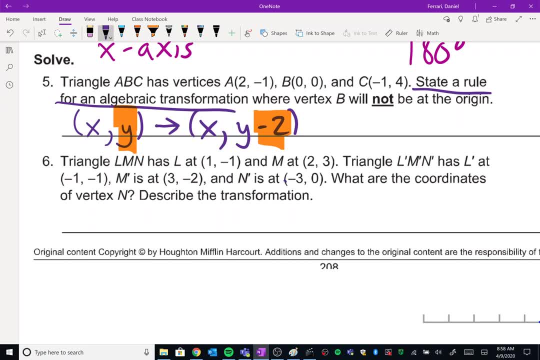 You can totally do this freehand, okay. Triangle LMN has L at one, negative one, M at two, three, okay, And you notice it didn't give us the coordinates for N. okay, That's gonna be what we're looking for in this problem. 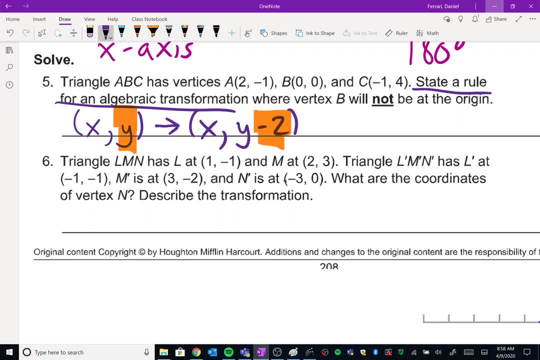 Triangle: L prime, okay, M prime and N prime. has L prime at negative one, negative one, M at three, negative two and N prime at negative three, zero. And we wanna find the coordinates of that missing point of the original point N. 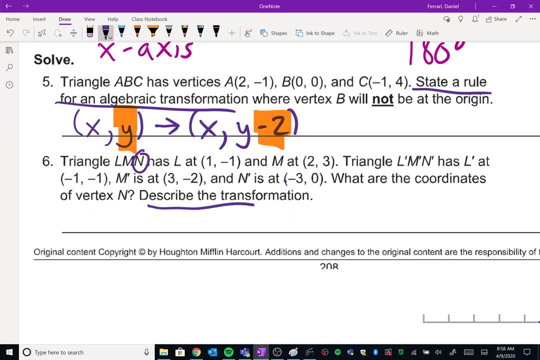 and then we wanna describe the transformation. Now, realistically, we're gonna probably describe the transformation before we do the coordinates of the vertex, because if we can't figure out what we're doing, it's gonna be pretty hard to tell where N should be okay. 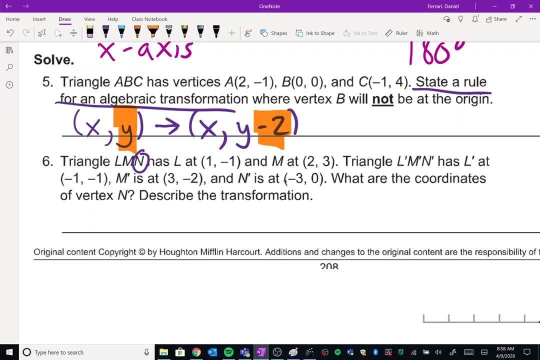 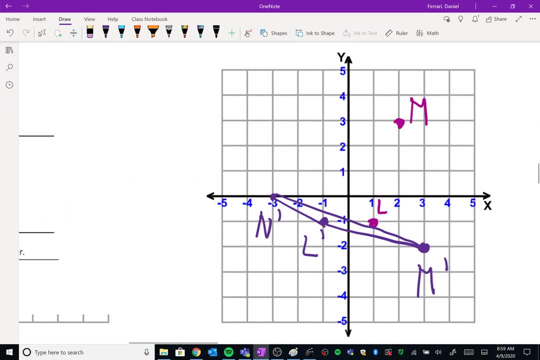 So again, this one is very hard to do if you aren't actually looking at the graph itself. So the first thing again I'd recommend is just graph it. okay, And so I did that. okay, So I plotted all the points. 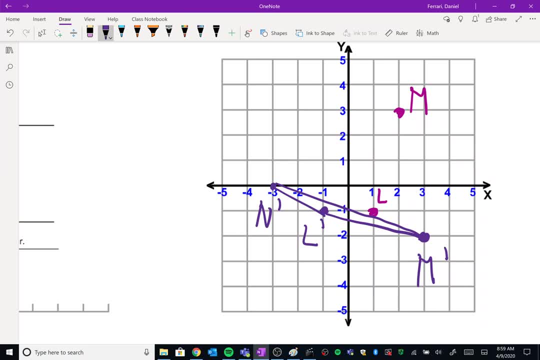 We have our N prime, L prime and M prime triangle, making this really thin, obtuse triangle, okay. And then we have, in the kind of lighter purple, the point L and point M, And again, our goal here is to find where this N prime point. 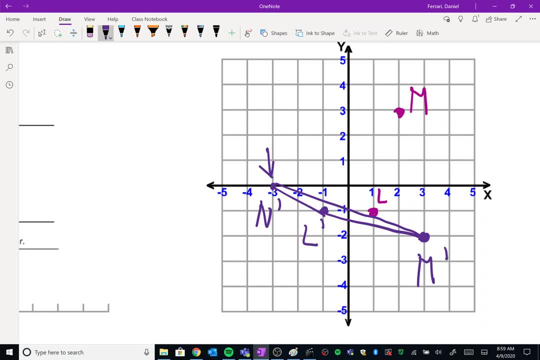 is gonna move where it moved from, to give us back that N that we started with, okay, And so, again, one thing we wanna keep in mind here is, because these are the primes, because the dark purple ones are prime, those are our final transformations. 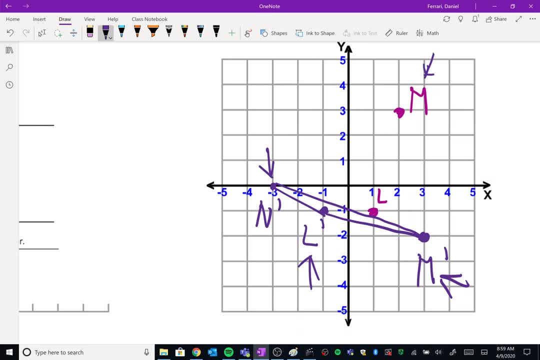 So we're starting- we essentially started- with the light purple and are ending with the dark purple. okay, So we wanna keep that in mind when we describe our transformation. Okay, so let's look at each point individually, okay, So for right now, I only want to look. 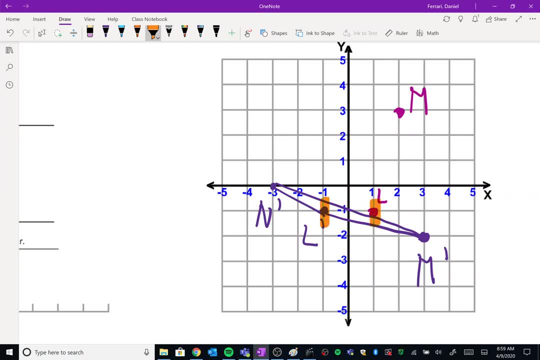 at my L's. okay, Because- and I'm gonna look at the other ones in just a second, but I wanna just use this to help me get started. okay, So it turns out that L is can be a little misleading if all I did was look at L, okay. 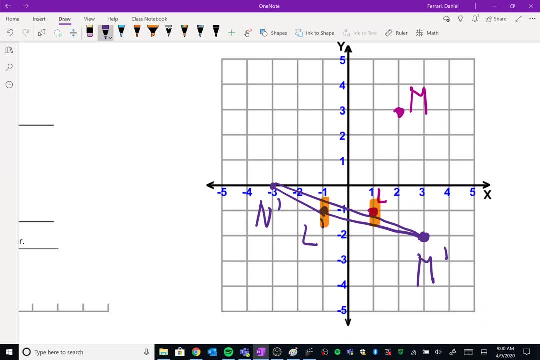 Because there are lots of ways to do this, okay. So, for example, I could do move L to L prime as a translation. I could take L and I would move it two units to the left and that would give me L prime. 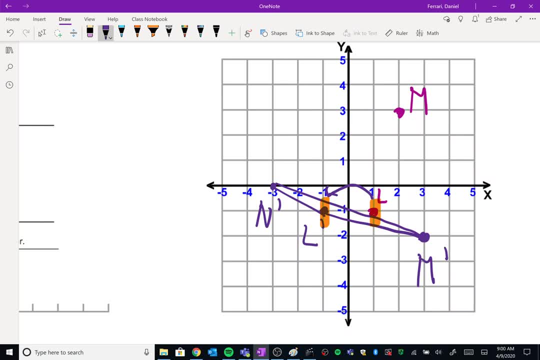 So that would be a case of a translation, okay, I could also reflect it over the Y axis, okay, And that would cause L to flip. oops, still in my highlighter, excuse me, That would cause L to flip and make L prime, okay. 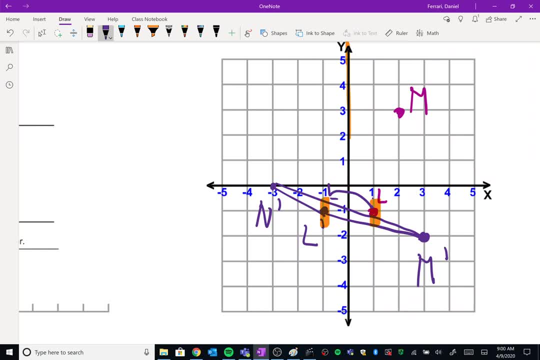 So I could do a reflection over the Y axis, okay, If all I was looking at is L. okay, I guess I should probably be writing these down. So we have a translation of two units left. potentially, We have a reflection over the Y axis, okay. 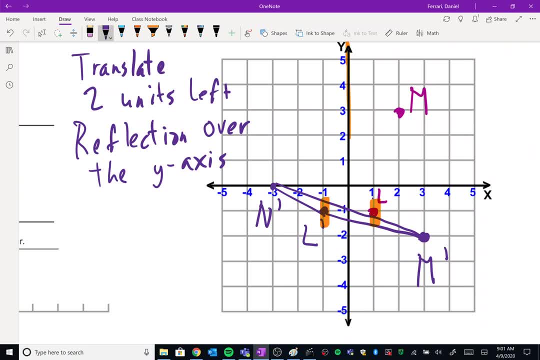 And then we can also do this as a rotation. okay, If I take point L and I rotate it now 90 degrees clockwise, okay, That will give me L prime. And if you don't believe me, take your paper and turn it 90 degrees clockwise. 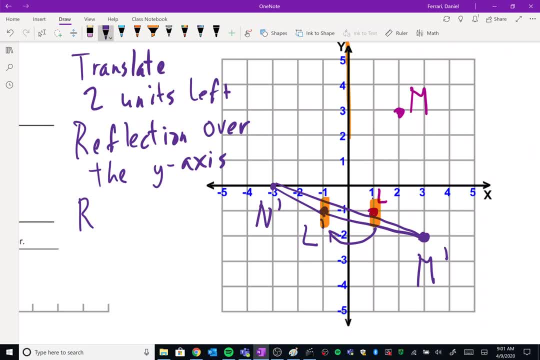 and you'll see exactly what I'm talking about. okay, So this one could also be a rotation of 90 degrees clockwise. okay, So we need to pick one of these three transformations, but only one of them can be the right answer. 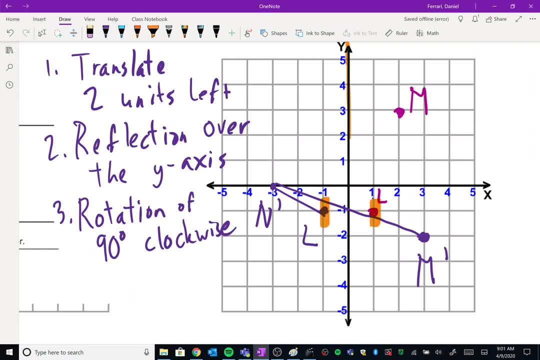 Okay, So let's go ahead and take a look at the other points now. Oops, guess I'm erasing everything. Okay, Let's look at the other points now and see if that will help. So now I am going to be looking at my other points. 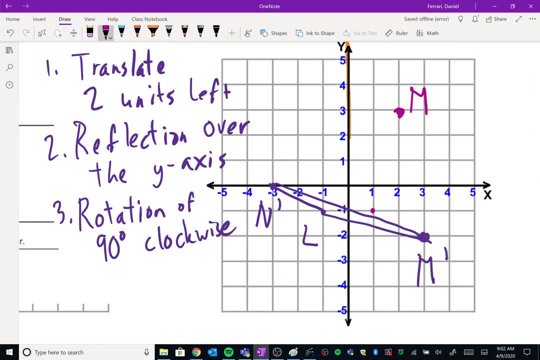 So I'm going to take a look at point M now, okay, And so let's do the exact same. let's do the same transformation, because if it worked for L, it should work for M. It should be the same transformation for all of the points. 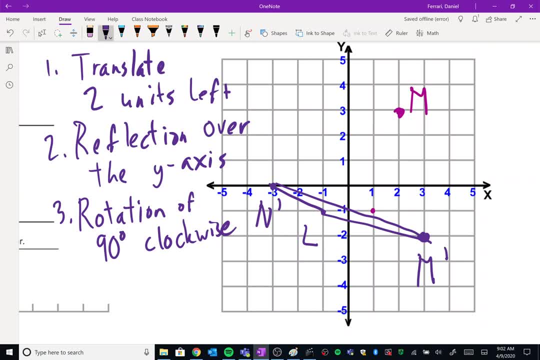 Okay. So if I take point M now, I'm trying to move it to M prime. Okay, Now if I go from point M and I translate two units to the left, okay, if I go two units left, that puts M prime over here. 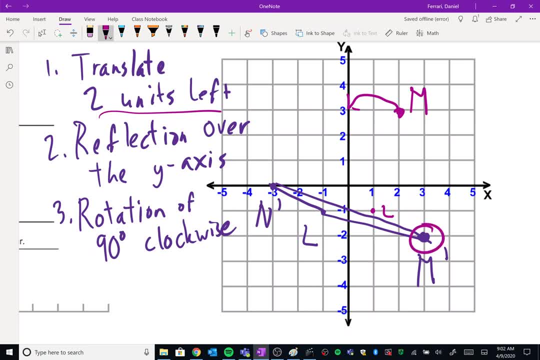 Okay, So obviously that is not where we want it to be, That is not down here with the M prime, So that means that number one cannot be the right answer. Okay, Then that puts us to number two, a reflection over the Y axis. 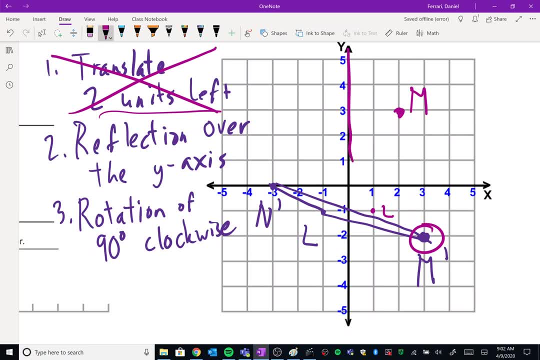 Okay, Well, if I'm reflecting over the Y axis, that would put M prime over here. Okay, And again, that is not where we want to be down in the fourth quadrant. Okay, So that means that one is out Now by process of elimination. we can probably maybe now, just know. 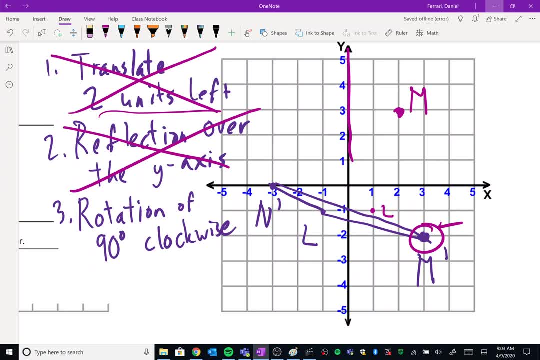 that it's going to be a rotation, 90 degrees clockwise. Okay, But it's probably worth us looking at it right And again, take your paper, turn it 90 degrees clockwise and you'll see that M rotates down and becomes M prime. 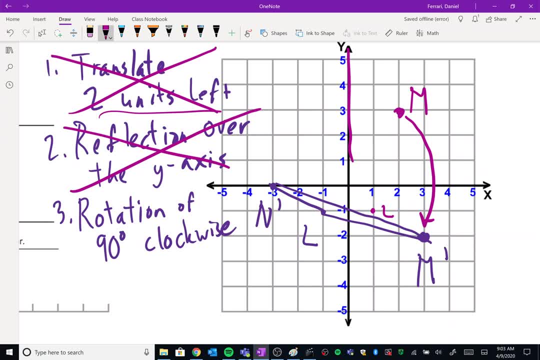 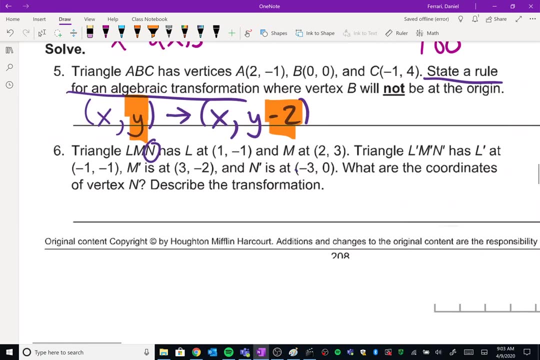 Okay, So that means that we must have done a rotation of 90 degrees: clockwise, Okay, And again clockwise because it's following, kind of how the clock normally moves, Okay, So well, we've done half the problem. now We've described the transformation. 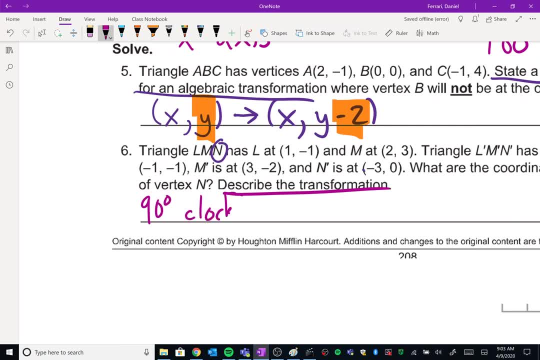 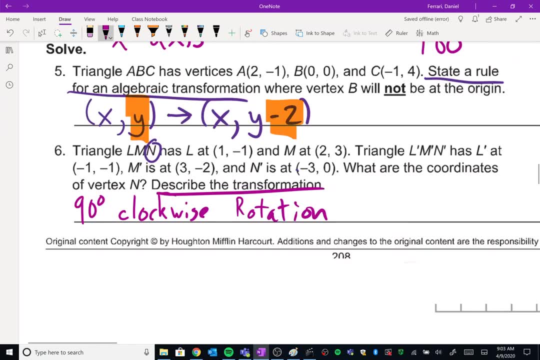 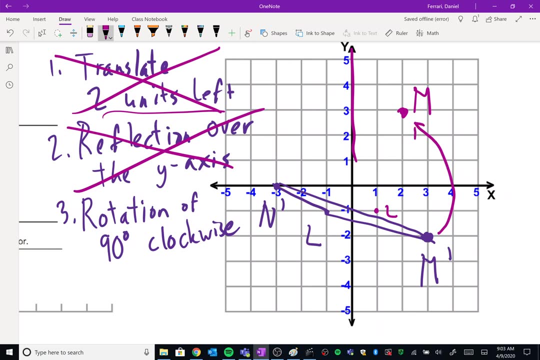 It's a 90 degree clockwise rotation. Now it's just a matter of figuring out where N was Okay. And so again, if we look at these now, I'm kind of working backwards. I'm going from the prime back to the original. 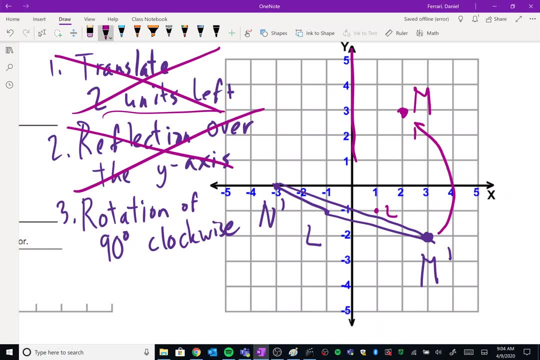 Okay. So essentially I'm reversing that rotation of 90 degrees clockwise by making a 90 degree counterclockwise turn. Okay, So that would mean that N prime take your paper, rotate it 90 degrees counterclockwise now. 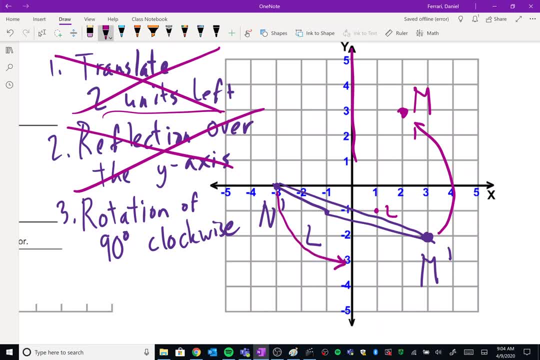 And you'll see that it will rotate to 0, negative 3.. Okay, So that means that that must have been my N, And again, if I connect these it might be a little bit easier to see, Okay, How those two shapes kind of turn into each other. 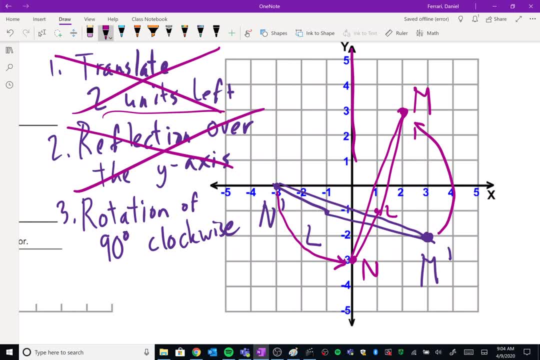 Okay, The purple shape. if you turn it 90 degrees, counterclockwise, right against what the original transformation would have been, you'll get back to what you started with in L, M and N. Okay, So let's look at the coordinates now. 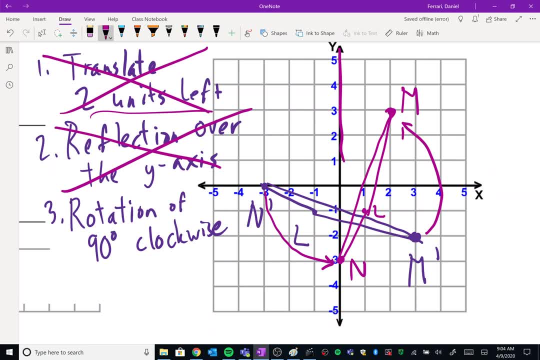 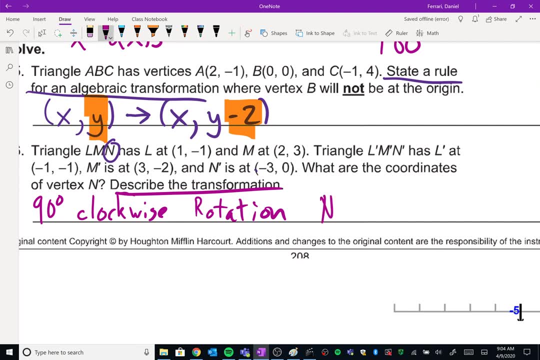 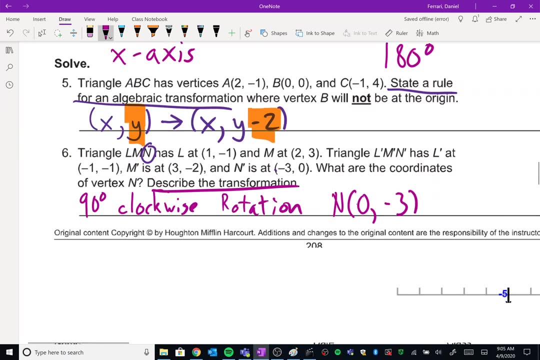 Again, this is going to be an X coordinate of 0 and a Y coordinate of negative 3.. So that puts us N is 0,, negative 3.. Okay, So that will do it for the C page. Now this is the hardest of all the pages, as I said at the start of the video. 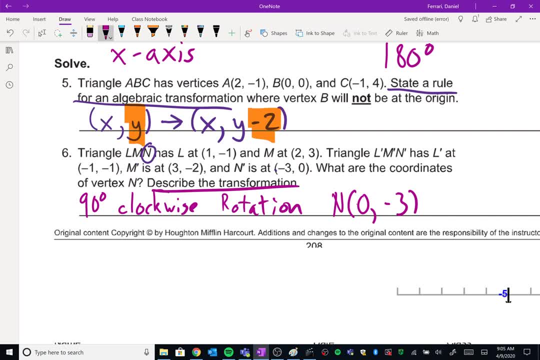 Okay. So when you go back and do A and B, this one should be a little more difficult, This one should be a little more straightforward. now, Use this as your model. And again I want to point out- I know I looked at it earlier-